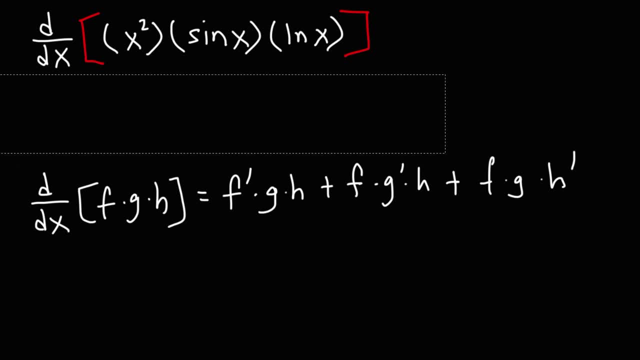 So at this point, what we want to do is identify what f, g and h are. So f is going to be. Let me write that here: f is going to be x squared, g is going to be sine x. 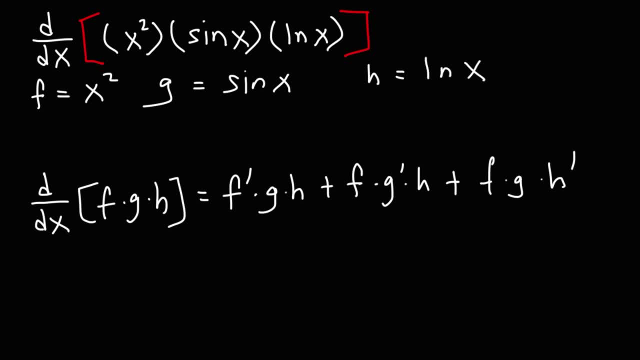 And h will be the natural log of x. So now let's find f prime. The derivative of x squared is going to be 2x. As for g prime, the derivative of sine is cosine. And as for h prime, the derivative of the natural log of x is 1 over x. 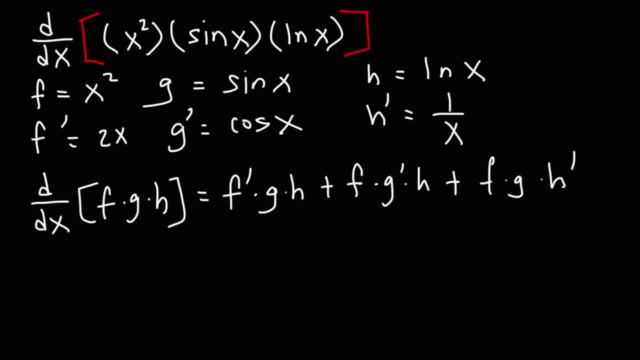 Now for those of you who might not know these things, if you need a review of derivatives, I'm going to post a link in the description section below where you can review the derivative of trigonometric functions, natural logs and how to use the power rule. 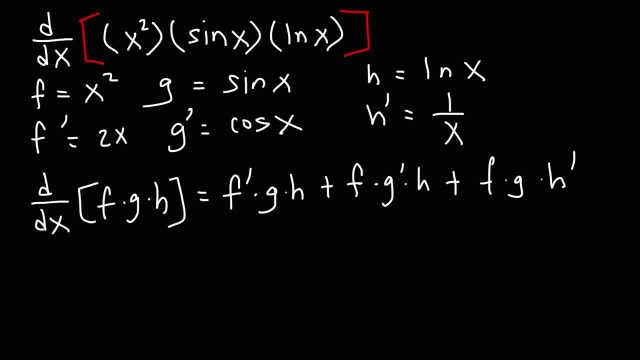 So feel free to take a look at that if you need to review that. But let's continue with this. So now all we need to do is plug in these values into this expression. So the derivative of this function is going to be f prime, which is 2x times g, which is sine x. 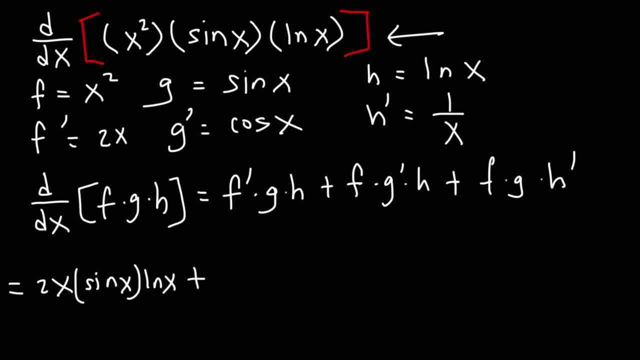 times h, that's ln x plus f, that's x squared times g prime, which is cosine x times h, which is ln x. And then we have f, g times h prime, which is 1 over x. 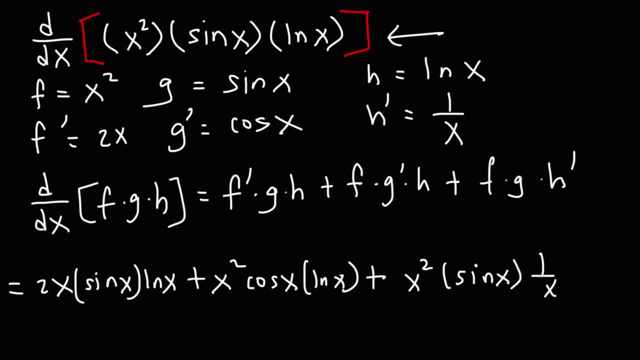 Now, this is our answer, but we can simplify it a bit: x squared times 1 over x, which is x squared divided by x, that's simply x. So this term reduces to x. The last thing that we could do is we can factor out an x, because we have it in each term. 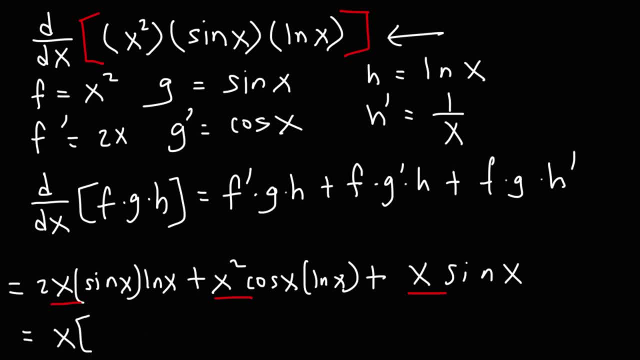 So, if we want to, we can write our answer like this: x and then times 2: sine x, ln x plus x, cosine x, ln x and then plus sine x, And that's as far as we can go with this problem.